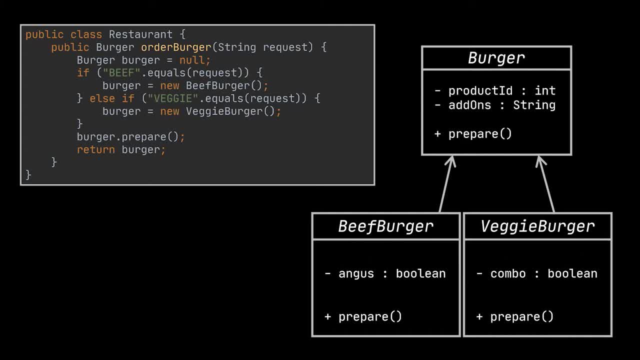 single class. what we can also do is extract the common behaviors of these products to this class, as they are already implementing them. Ok, our application looks complete now, but when we see code like this, we know that when things change, like if we add new recipes to our delivery menu or more products to our 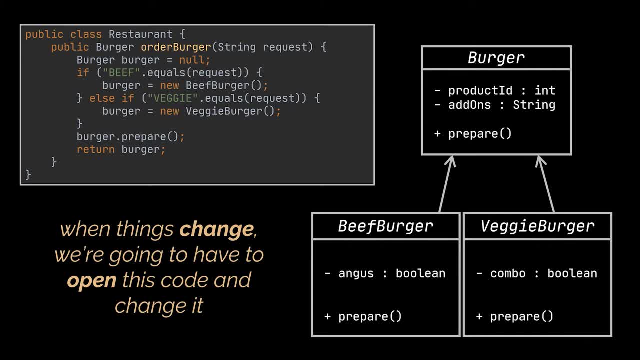 restaurant, we're going to have to open this code and change it, and that violates our open, closed and single responsibility principles. We'll also end up writing the same piece of code in several places in the app, making things even worse. 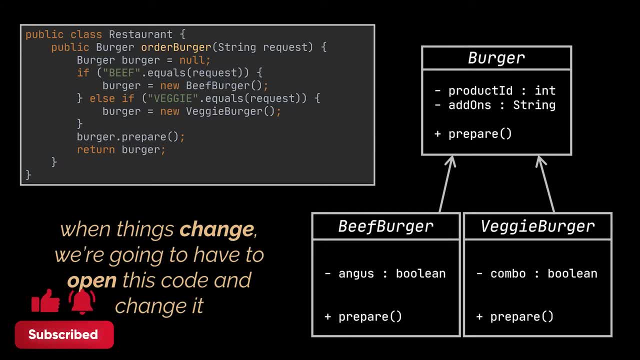 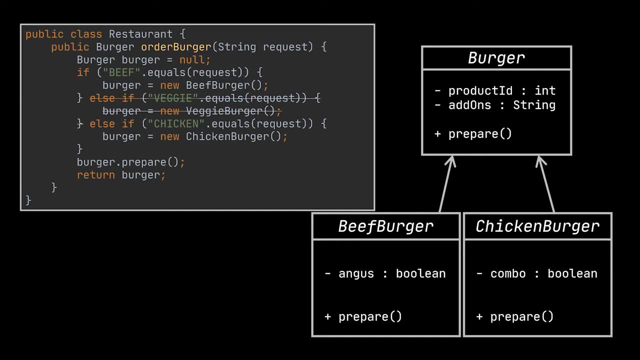 So what do we do? Well, let's look at what varies and encapsulates it. When our restaurant grows and changes over time, we are going to add and remove recipes from the menu. So in the second version of our app, we removed the veggie burger and 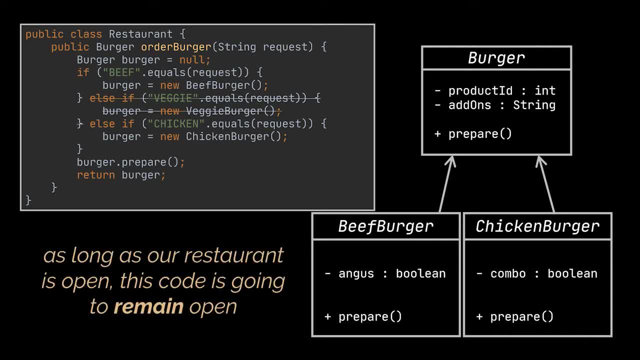 added the chicken burger option. You can clearly see that the variety of food that we are adding to our menu is changing over time. The amount of food we can deliver is getting in the way of closing this code for modification and, as long as our restaurant is open, this code is going to remain open. 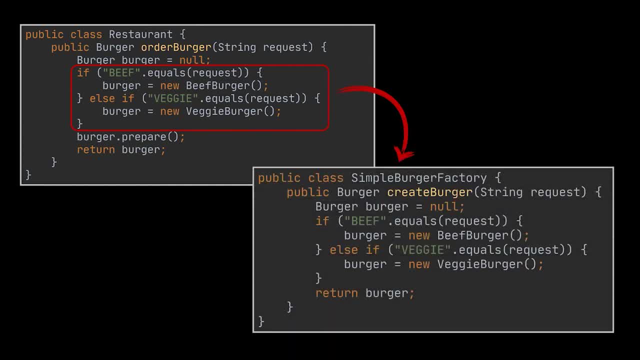 To fix this. what we do is take our burger's creation code and encapsulate it, separate it into a class called a factory. Why a factory? Because this is a class whose sole responsibility is creating burgers. It's a burger factory. Now, anytime we want to order something from our restaurant, we'll call this method pass. 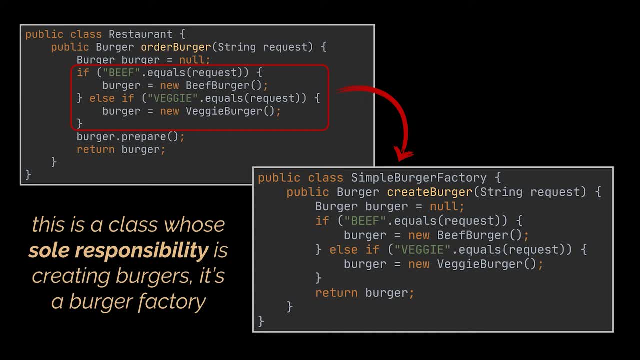 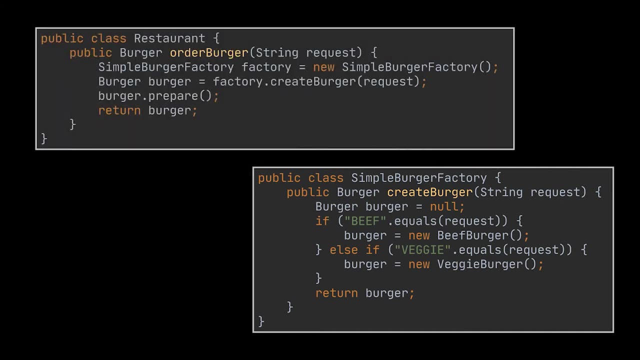 a type and, after figuring it out, the method will return the requested order. for us that implements the burger class. Now all this code is in one place, nicely separated from the rest of the restaurant code, And to integrate it back in our original method, what we have to do is create a factory object. 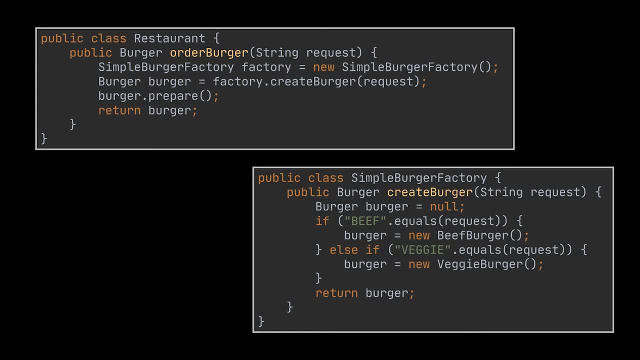 pass to it the type and boom, our food is ready. Our order burger method no longer has to worry about the concrete type of the burger requested, because, whatever it is, we know that it will implement the burger itself. So let's go back to our original method. 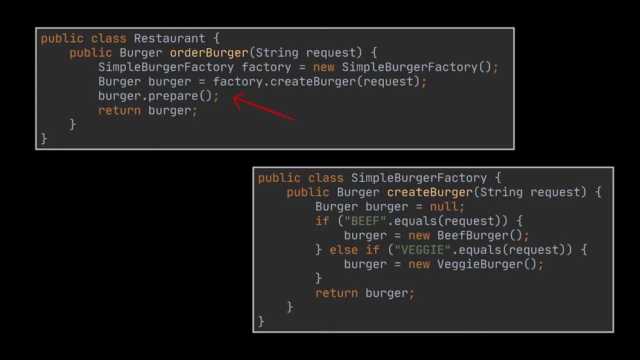 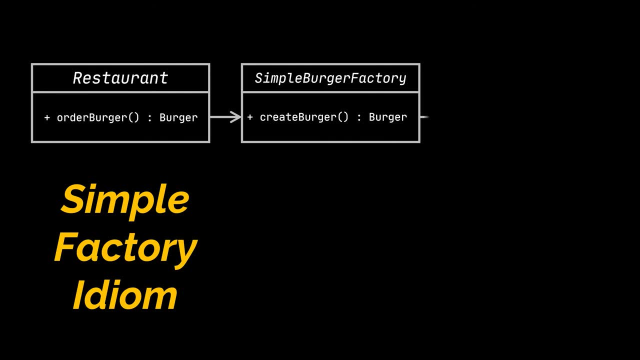 We call this design the simple factory item, and our example can be represented by the class diagram you see in front of you. It starts with the client of the factory, in our case the restaurant class itself. Then we have our factory, which is the only place where the concrete type of burgers is. 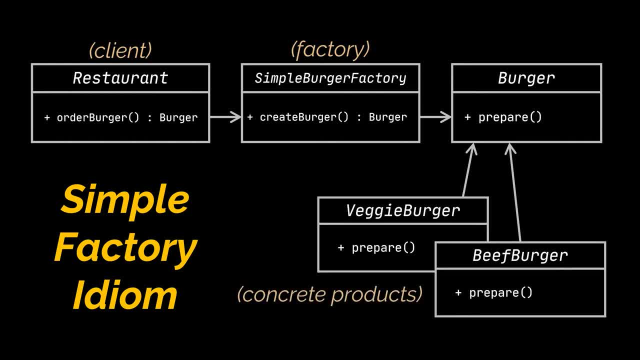 known. And then we have our concrete products, the burgers our restaurant delivers via the app we are implementing. All concrete products must implement the same interface or abstract class. Now, one thing to note is that the simple factory we've been discussing since the 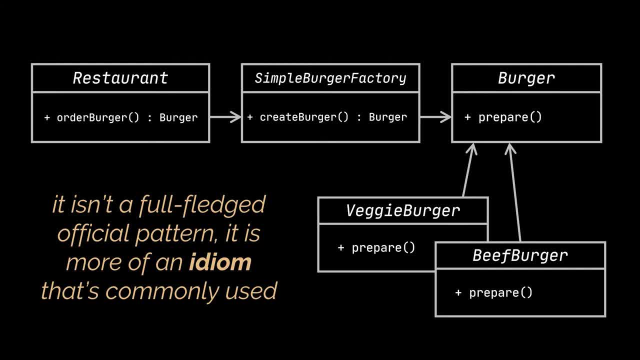 beginning of this video is not a full-fledged official pattern. It is more of an iGEM that's commonly used. However, it is the first step in understanding one of the most powerful design patterns out there: the factory method design pattern. 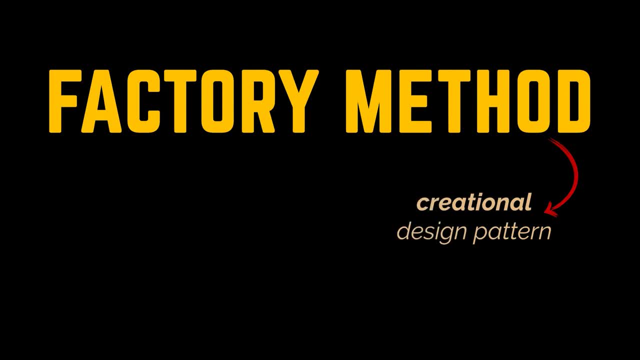 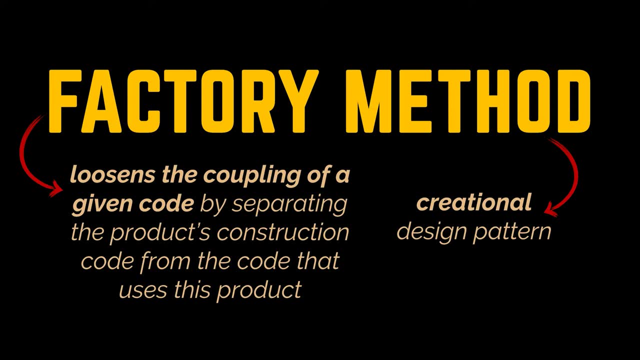 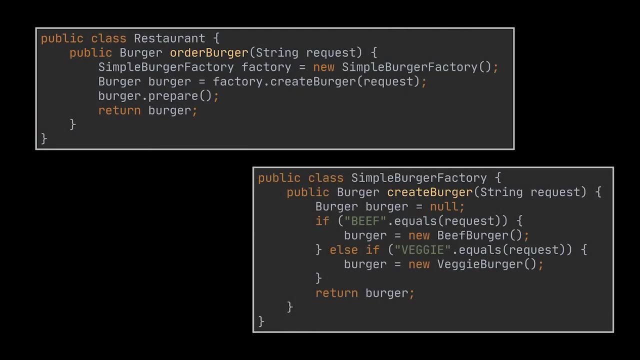 This pattern is a creational design pattern. It loosens the coupling of a given code by separating the product's construction code from the code that uses this product. In our previous example, the product was the burgers we are delivering. So let us go back to this example to try and see together why the implementation we did. 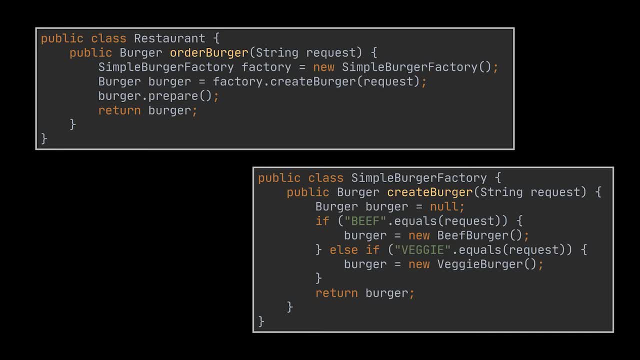 isn't considered a full-fledged design pattern. When we encapsulated the creation logic of our burger in the simple factory class, we isolated this logic and created a class whose sole purpose is creating burger objects. By doing this, we followed the single responsibility principle, and that's great. 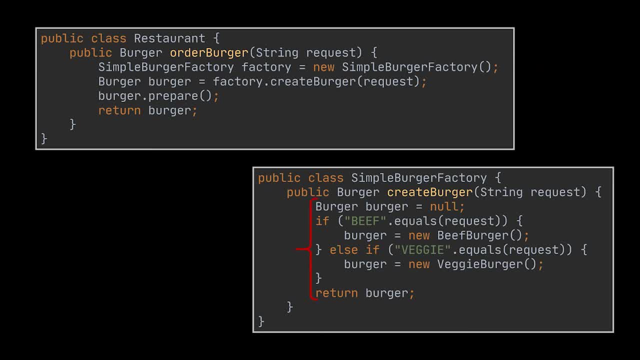 However, if you look closely, you will see that this is a single responsibility principle. However, if you look closely, you will see that this is a single responsibility principle And that this class on its own is still open for modification, And when we add more recipes to our menu, we will have to add if statements to this. 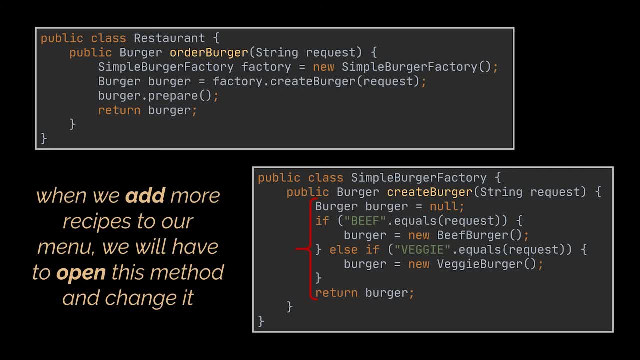 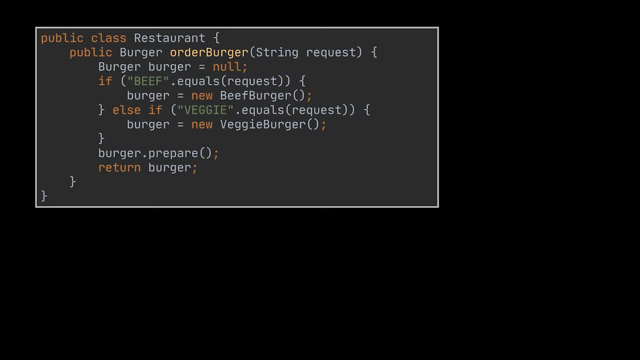 method, And one way to fix this is by applying the factory method design pattern. To do that, let's remove our simple factory class and put back the creation logic and the order burger method inside the restaurant class to start from scratch. Okay, the first thing we need to do is abstract the restaurant class. 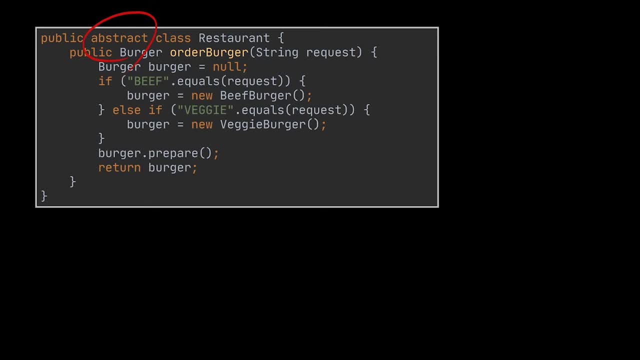 Why are we doing that? Well, it's because the createBurger method that used to exist in the simple factory class- simple factory we had- will now become an abstract method inside the restaurant class. This method is the factory method and will be implemented by the subclasses of the restaurant. 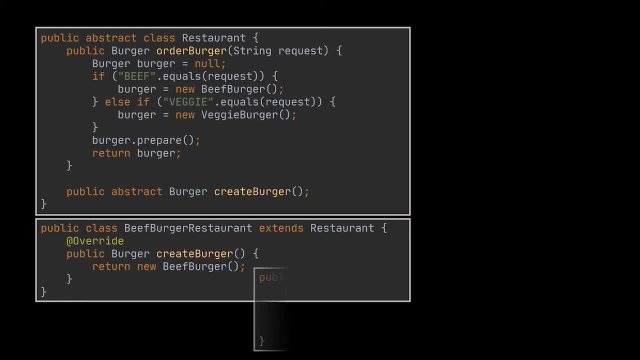 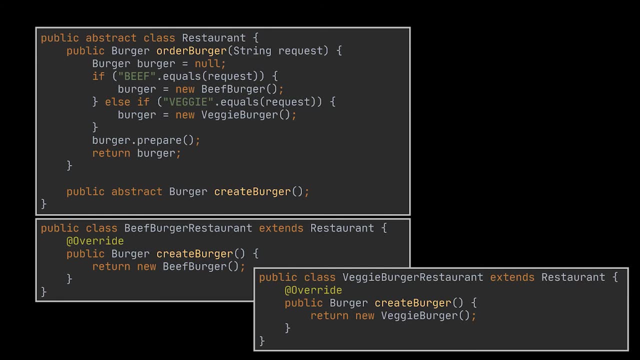 class. In this example, and based on the burgers we are delivering, these subclasses will be the beef burger restaurant and the veggie burger restaurant. You see, that is actually how you pinpoint the usage of a factory in a given code. As the factory method design pattern relies heavily on inheritance, it delegates objects. 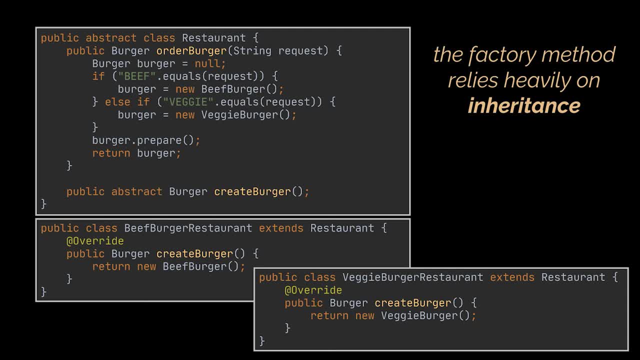 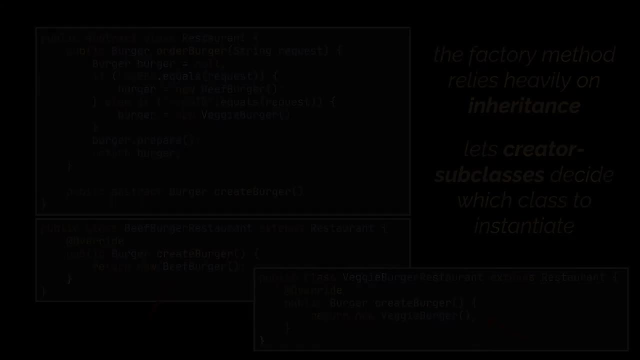 creation to subclasses that implement the factory method. So, after defining an interface for our products, in this case the burger interface, we let creator subclasses decide which class to instantiate, and that is exactly what we are doing in this implementation. Ok, now all that is left to do is replace the creation code inside our business logic. 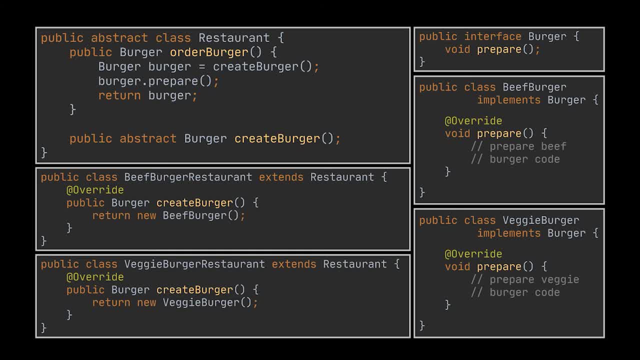 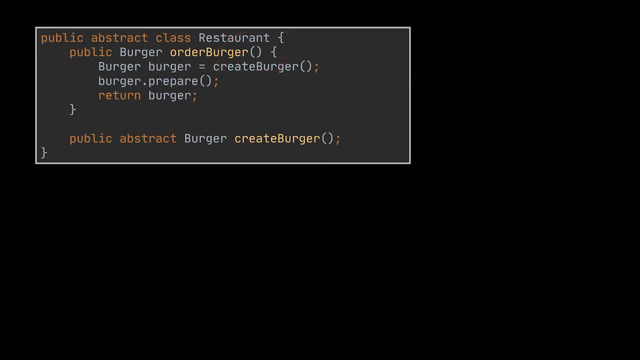 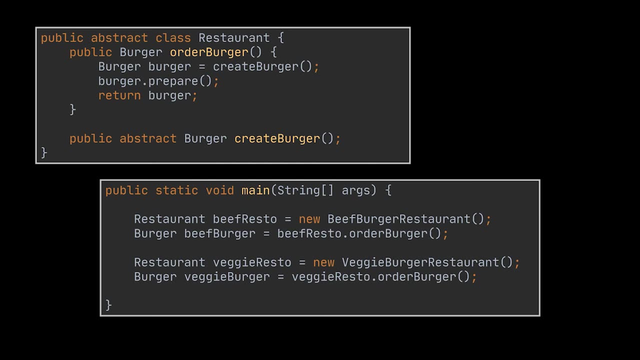 or the order burger method with the factory method. Notice that the order burger method is no longer dependent on the request object, and that's because we don't need it, As the users of our restaurant can now directly instantiate and invoke the concrete restaurant class implementation they need, and the correct prepared burger will be returned to them. 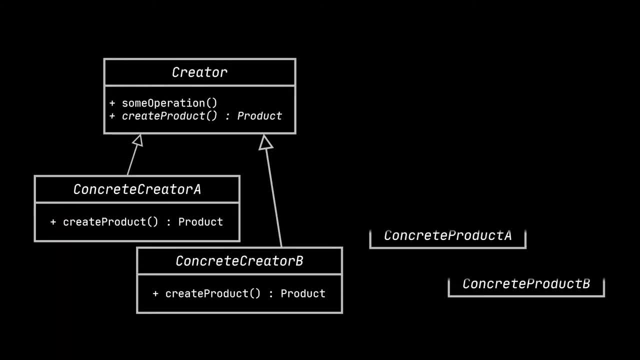 Now I want you to take a look at the structure of the factory method pattern, represented using a UML class diagram, as you may encounter it while going through different references. Let's try to relate this structure to our delivery application example. The product interface and the concrete products obviously represent the burger classes in 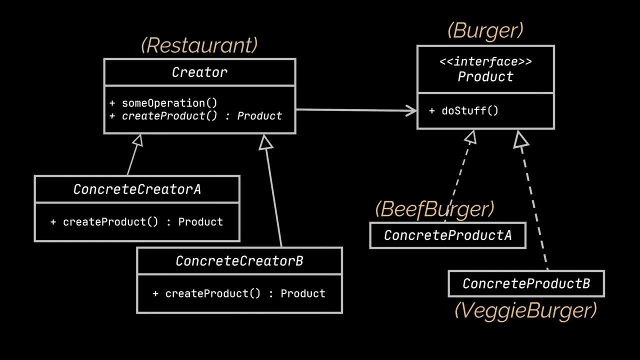 our example. The creator class, however, the one housing the factory method, was represented using the restaurant class in our example. And finally, the concrete creators are represented by the different restaurant classes in which the creation process of our burgers is defined. Ok, now you know how to implement the factory method pattern, but when should you use this? 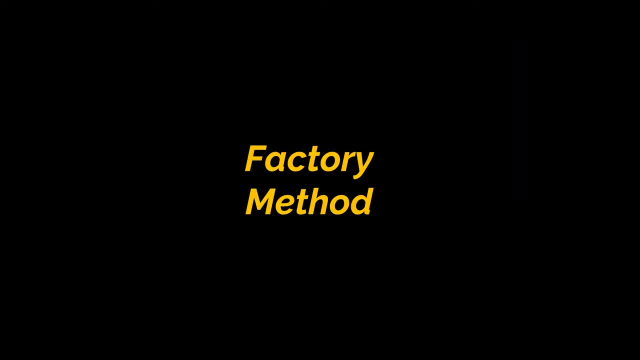 pattern. Should you apply it on all parts of your application that have to do with creation stuff? Well, if you have no idea beforehand of the application, then you can use the factory method pattern. If you have no idea beforehand of the exact types and dependencies of the objects, your 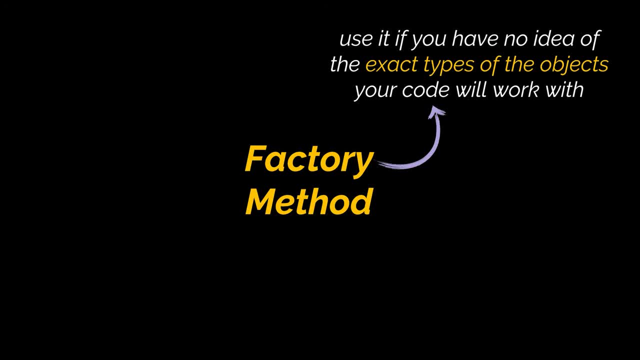 code will work with, then it is probably a hint that you should make use of this pattern right from the beginning, As the factory method makes it easy to extend the product construction code independently from the rest of the application and hence allows you to introduce new types of products. 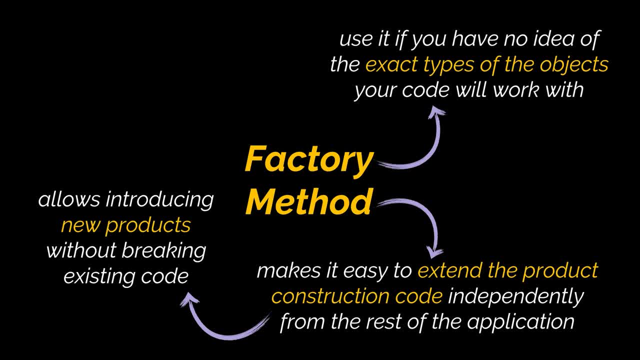 into the program without breaking existing client code. by doing this, you wouldn't only be providing the users of your application with a way to extend its internal components, but also, And most importantly, you will be following and applying the open-closed principle, and. 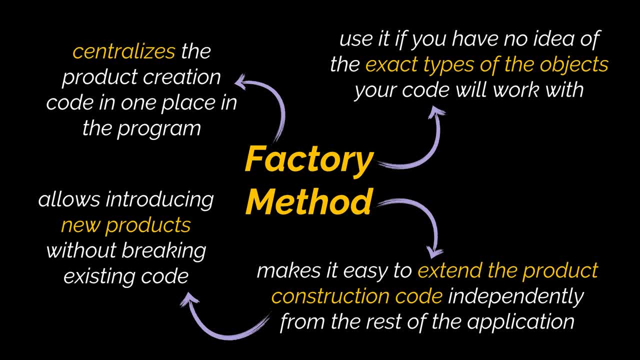 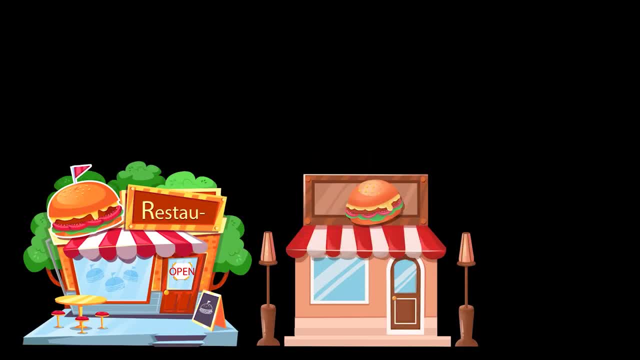 the single-responsibility principle, as you are centralizing the product creation code in one place in the program. Now, before ending the video, I want you to imagine that your burger business boomed and you decided to open another restaurant. This restaurant will deliver the same burgers you have. however, this one will prepare them.